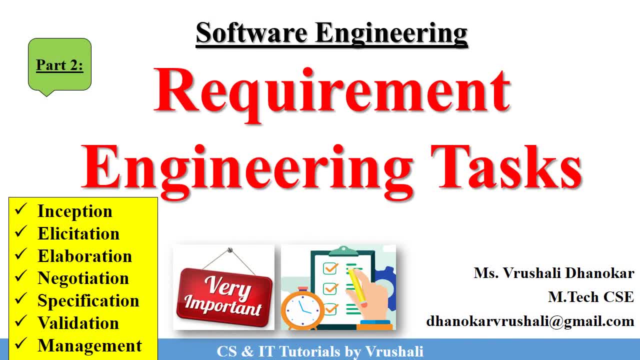 Good evening everyone. This is Rishali. In previous sessions we discussed about requirement engineering and how to establish groundwork. in part 1 video I have mentioned complete software engineering subject playlist link in below description box. Now in today's session we will discuss about the next important point, that is, part 2, requirement engineering. 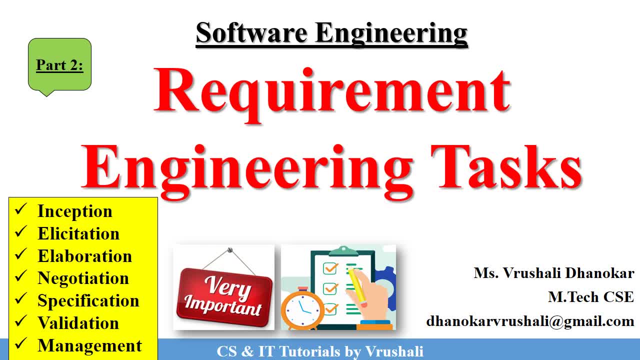 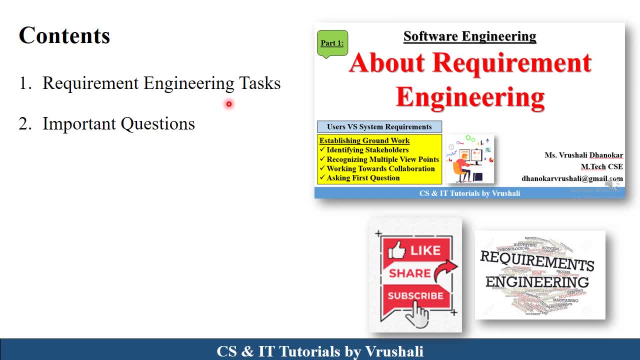 task. As per your exam point of view, this is one of the most important question. Let's start the session. In this session we will discuss in detail requirement engineering task and some important questions that have asked in previous year question papers Now. 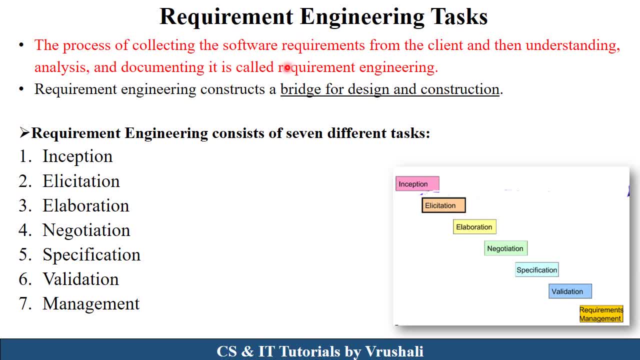 the first thing is what exactly requirement engineering? We already discussed this thing in detail in previous sessions. Basically, requirement engineering is a process of collecting all the software requirements from the customer, After that understand those requirements, analyze those requirements And document it properly. This is called as requirement engineering, So requirement. 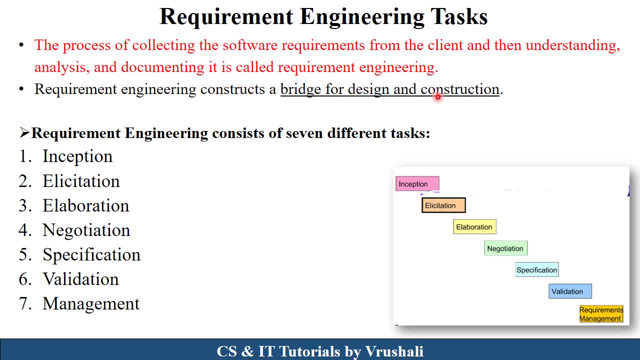 engineering, construct a bridge for design and the construction phase. Now, in software engineering, in requirement engineering, there are seven different tasks, sequentially like inception, elicitation, elaboration, negotiation, specification, validation and, at the last, management. Now let's discuss all these tasks in detail. 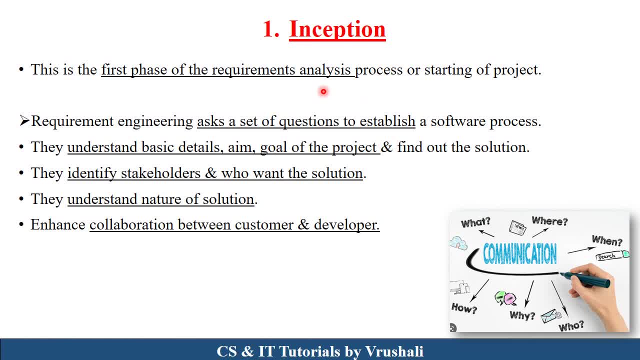 Now the first phase of requirement analysis and the first task in requirement engineering is inception. As we know, in software development life cycle, the first phase is requirement gathering and analysis. There is a communication between the customers and the project head and development team. Basically, there is a communication between all the stakeholders. 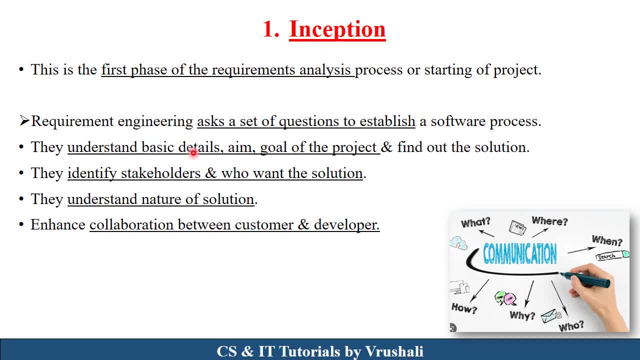 Now this inception task focus on the basic detail about the project. For example, customer want online shopping application- We have already talked about this, But basically shopping application. So here they understand what is the aim of the project, What is the goal of the project and what is the future of the project. means they understand. 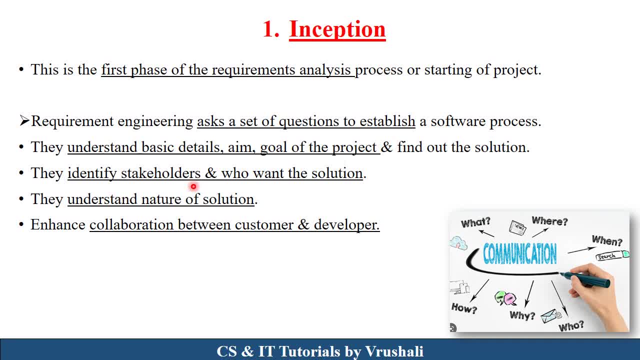 the basic details also here. they identify. stakeholders means which type of people included in the project like, which type of customers here, which type of organizations here and which type of developer, tester as per skill, included in the project. So identifying stakeholder is one of the most important thing. after that, they also identify. 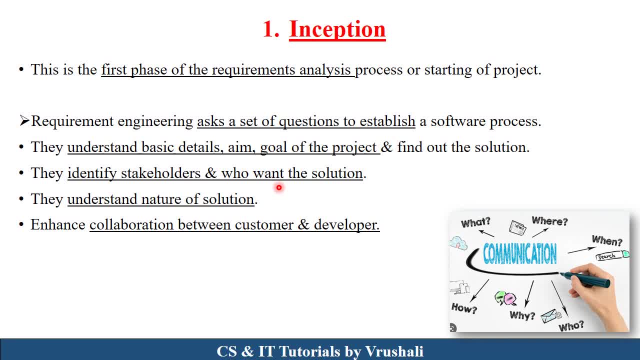 who will be the user of this project? suppose customer want online shopping application, So which type of user use those project? so they identify this kind of thing, then they also understand nature of the solution. for example, a particular project is regarding to the banking application, regarding to the reservation, regarding to the college management. 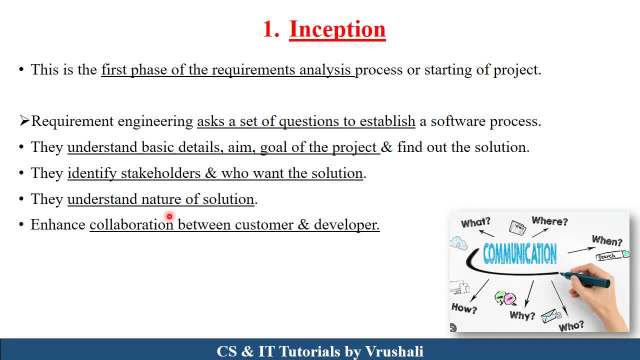 So they understand nature of the problem And find out the solution as per the problem. basically, due to inception task, there is a collaboration between customer and developer means there is a strong communication and strong bonding between customer and developer. So, basically, inception task focus on the basic details about the project. next, now the next. 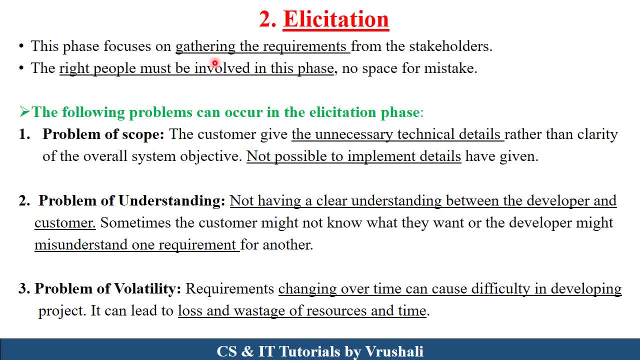 and second task is elicitation. So elicitation phase: focus on gathering the requirements here right people involved in this phase. Suppose you have collected wrong requirements then your project will not work. and if we have collected right requirement then your project will be generated accurately and quality. 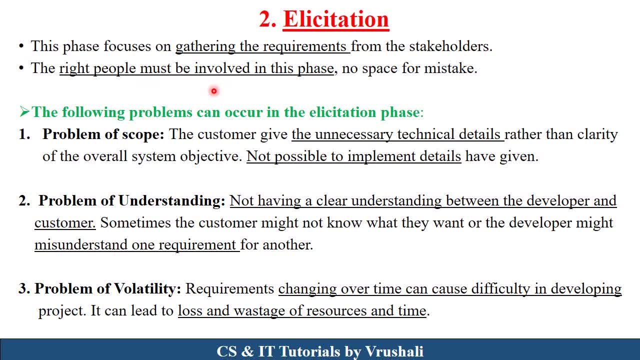 right. so that's a right people involved in this project. now, which type of problem occurs in elicitation phrase? as per your exam point of view, this is one of the most important question, like which type of problem occur in elicitation phase. So basically, there are total three type of problem. 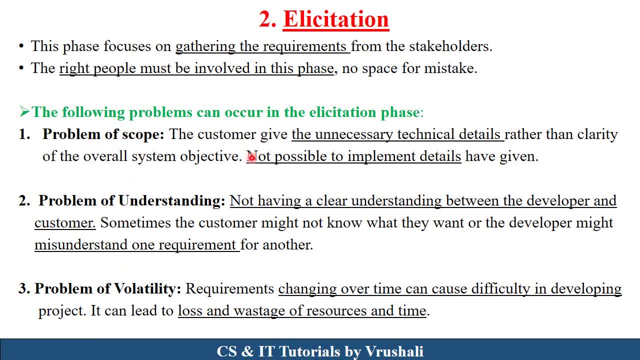 The first problem is problem of scope. means sometimes customer give unnecessary technical details about the system, or sometimes customer give the particular idea which is not possible to implement. So this is called as problem of scope. Now the problem of understanding: sometimes customers are not not clear about their idea. 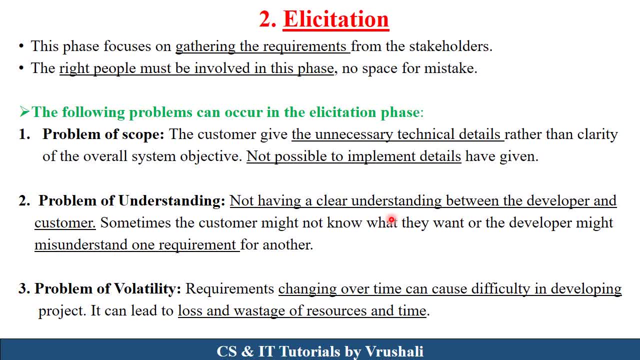 about the requirements. that's why there will be misunderstanding generate between customer and developer. So there is a problem of understanding. and last one is a problem of. volatility means customer requirements are continuously changing. that's why it is very difficult to develop a particular project. that's why there is a loss of and wastage of resources and time. 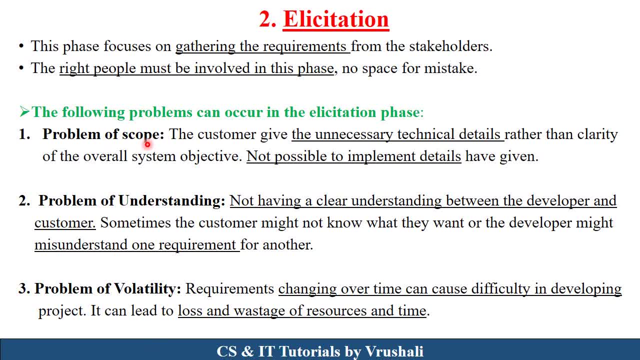 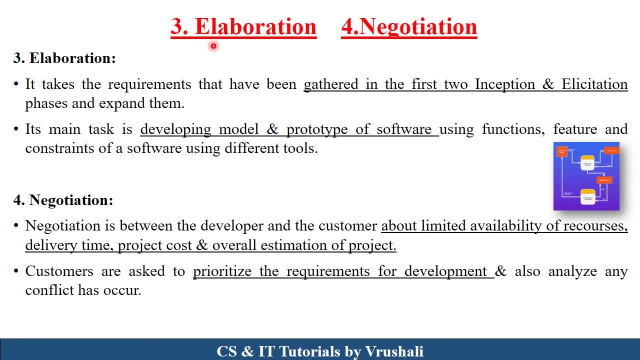 So basically these three problems occurs in elicitation: problem of scope, problem of understanding and problem of volatility. next, now, the next and third task is elaboration. So basically, Elaboration means they gather all the information from the first two phases: from inception phase they gather basic details and from elicitation phase they gather clear idea and clear requirements. 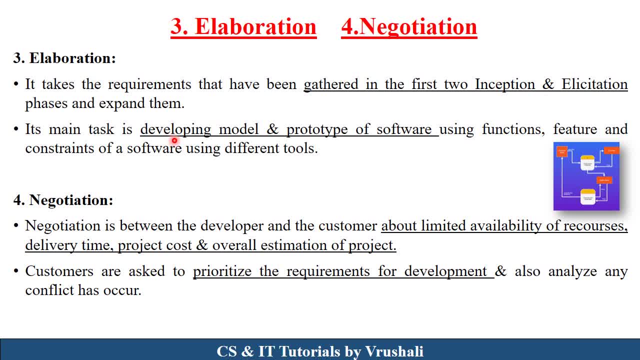 after collecting clear requirements here in elaboration phase they develop a rough model or prototype. prototype is not actual model. this is just a rough idea. means what exactly customer want. after developing prototype as per the functions, features and requirement, They take a suggestion from the customer. if customer want any changes, they do this changes. 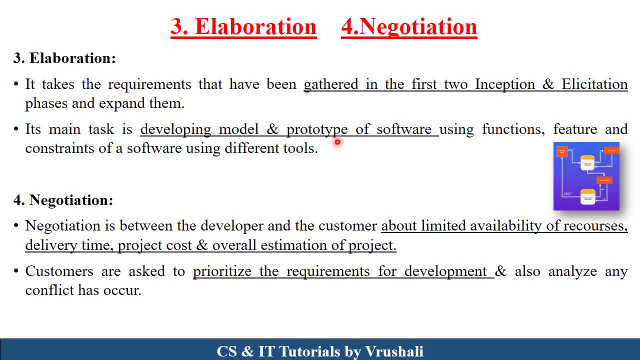 in prototype and after customer satisfaction they develop a actual product right. so this is a elaboration phase here, develop a model or prototype now. next one is a negotiation. so there is a negotiation between developer and customer. customer negotiate with developer regarding project cost, regarding delivery time, suppose. sometimes customer want project. 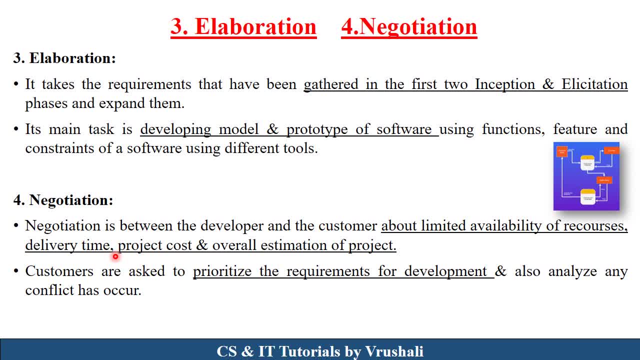 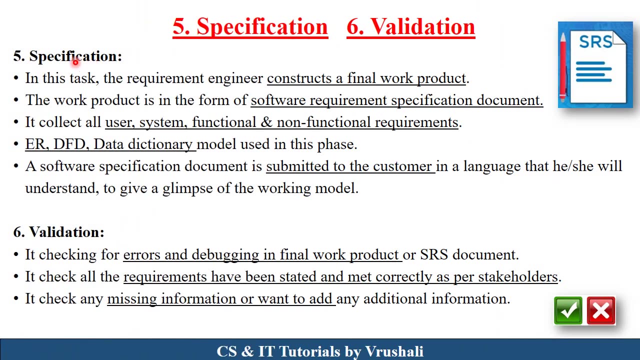 early. so they negotiate with the developer right now. they also negotiate with some available resources. sometimes customer want some prioritize requirements right. sometimes they want a particular requirements quickly. they want to release a product in market quickly. so this kind of negotiations are done in this negotiation task next now. the next one is a specification. 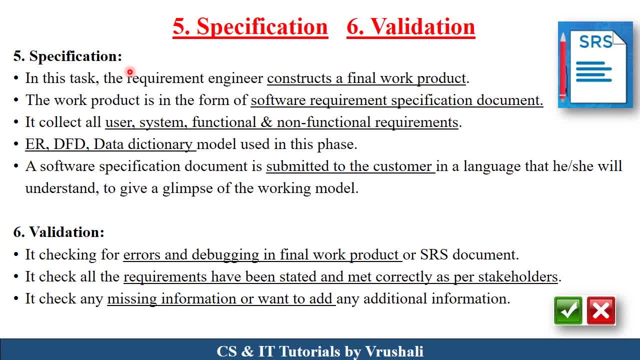 so after completing all this first task, Now there is a specification means here: requirement engineer, construct a final work product. final work product means SRS document. SRS means software requirement specification. this is a one kind of document where all type of requirement from the customer like user requirement system. 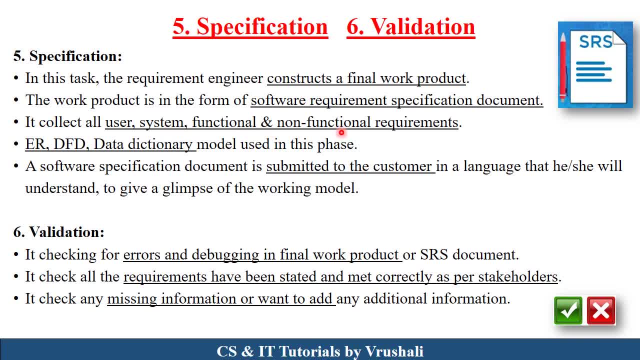 requirement, functional and non functional requirement. this- all types of requirements are collected and mentioned in the document accordingly. so this document is called as SRS document here. in this document also ER diagram, DFT diagram, data dictionary diagram- also have mentioned that will be understandable by the customer. now this SRS document after: 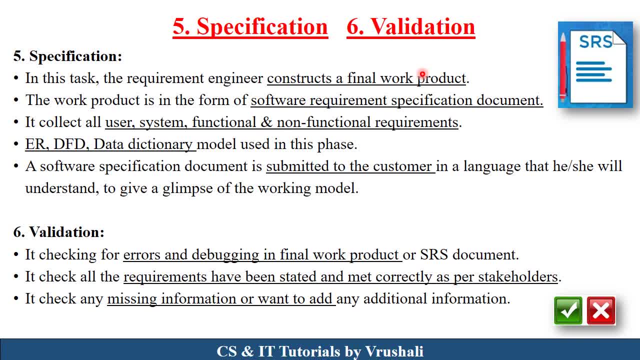 gathering all the requirement, analyzing the requirement and mention all this requirement into the document. now this document is submit to the customer. so this document are mentioned in the language that will understand by the customer as per their working model. clear and last one is a validation. so after submitting document to the customer, it validate the. 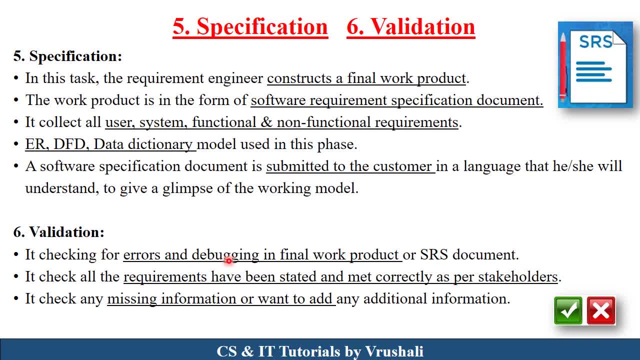 document means it check that if there are any errors are there in this SRS document or final work product, or if there are any requirements that have correct, not correctly mention or that have some, there are some additional requirements are there. so it check all this thing. they also validate some missing information is there in this particular document, so validation. 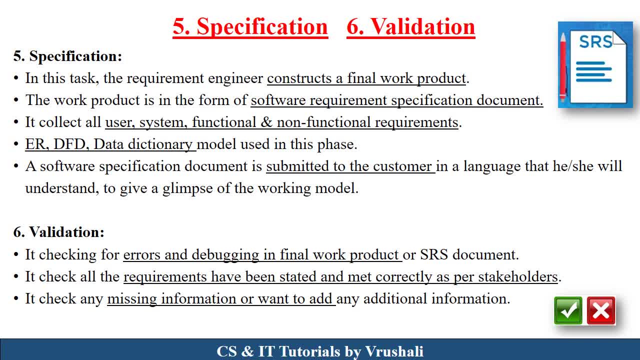 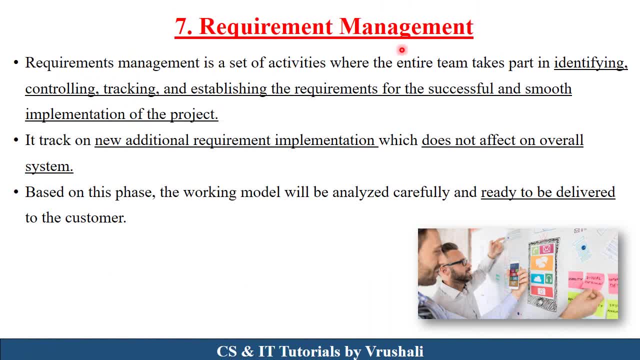 basically means test a particular document whether it is as per the customer requirement or not. clear. next now, the next one and last one is a requirement management. so basically, requirement management handle all the changing requirements. ok, here the management team identify, control, track and establish all the requirements. 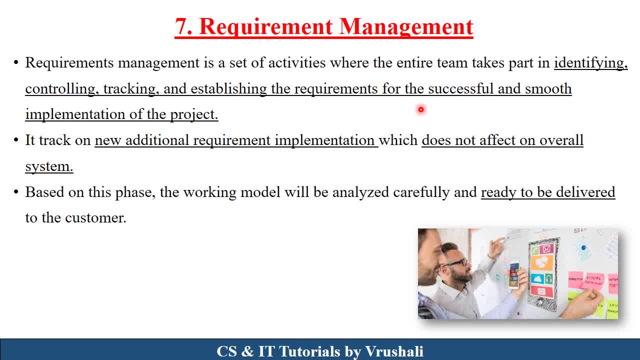 and they also check that your project and your product is developed as per the customer requirement or not. and if there are some new, additional or changing requirements, then they check all the requirements from the customer. so they check that whether it is this particular requirement does not affect on overall system, right? so after managing all this requirement, 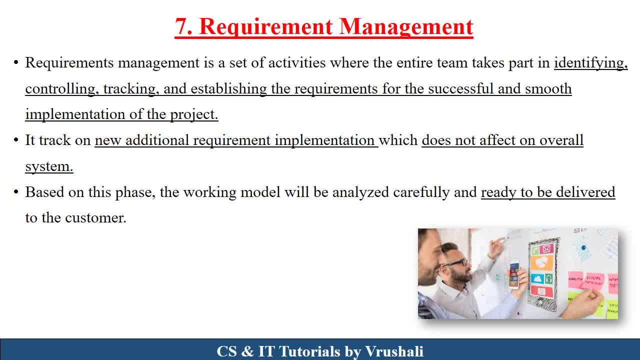 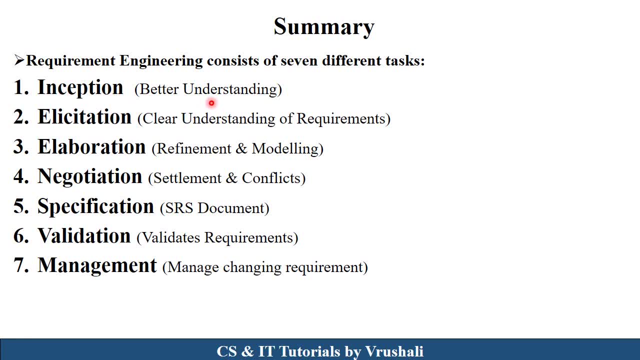 they ready to deliver the product to the customer. clear next, basically, what we learn in this session. the first task is a inception task. there is a better understanding and basic understanding about the project. elicitation means clear understanding, clear requirements about the project. Elaboration means modeling.